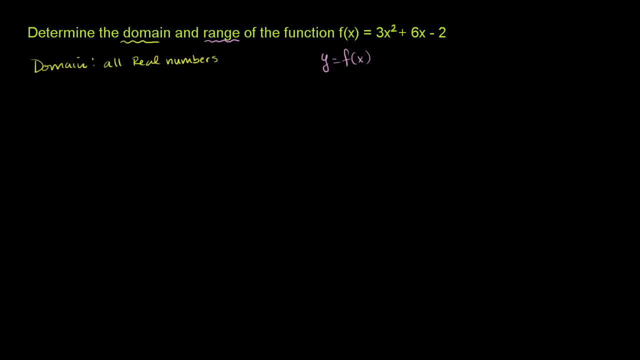 going to try to graph this function right over here, And if you're familiar with quadratics- and that's what this function is right over here- it is a quadratic- you might already know that it has a parabolic shape, And so its shape might look something like this: 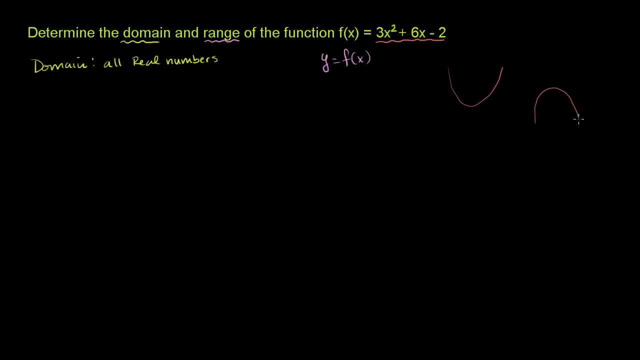 And actually this one will look like this. It's upward opening. But other parabolas have shapes like that And you see, when a parabola has a shape like this, it won't take on any values below its vertex when it's upward opening. 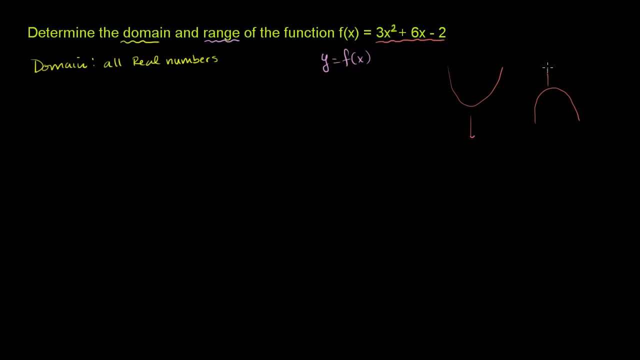 And it won't take on any values above its vertex when it is downward opening. So let's see if we can graph this and maybe get a sense of its vertex. There are ways to calculate the vertex exactly, But let's see how we can think about this problem. 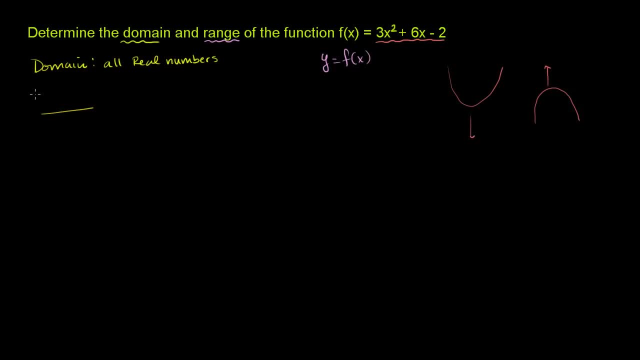 So I'm going to try some x and y values. There's other ways to directly compute the vertex. Negative b over 2a is the formula for it. It comes straight out of the quadratic formula which you get from completing the square. 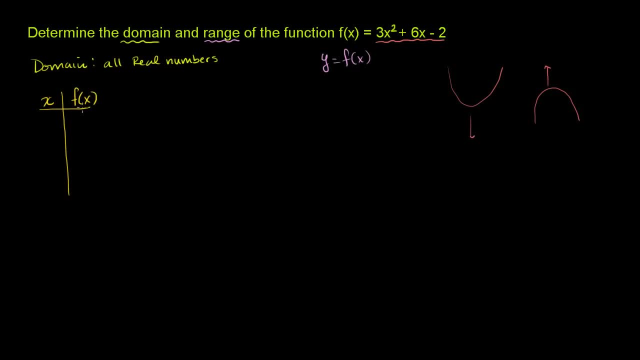 But let's try some x values And then let's see what f of x is equal to. So let's try well the values we've been trying in the last few videos. What happens when x is equal to negative 2?? 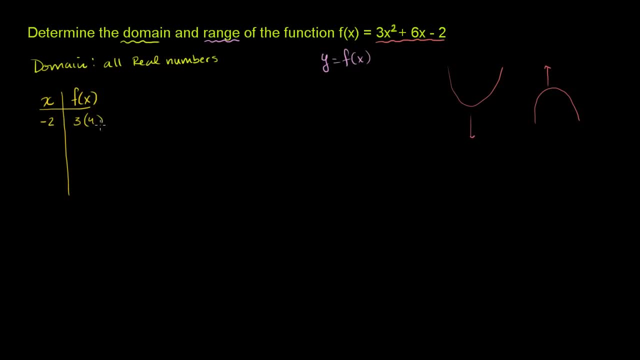 Then f of x is 3 times negative 2, squared, which is 4, plus 6 times negative 2,, which is 6 times negative 2.. So it's minus 12 minus 2.. So this is 12 minus 12 minus 2.. 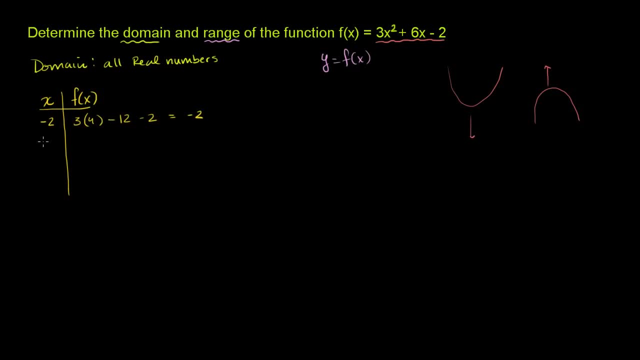 So it's equal to negative 2.. Now what happens when x is equal to negative 1?? So this is going to be 3 times negative 1 squared, which is just 1.. Minus, Or I should say plus, 6 times negative 1, which is minus 6.. 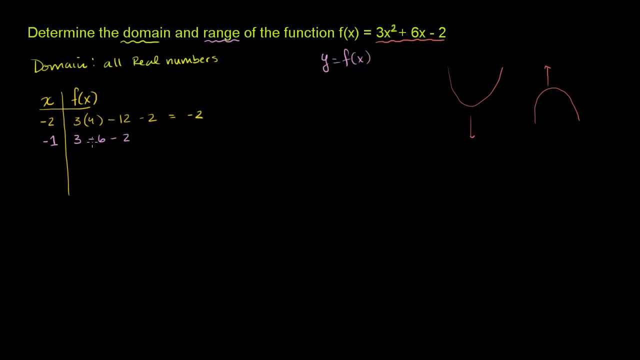 And then minus 2.. So this is 3 minus 6 is negative 3.. Minus 2 is equal to negative 5.. And that actually is the vertex. And you know the formula for the vertex, once again, is negative b over 2a. 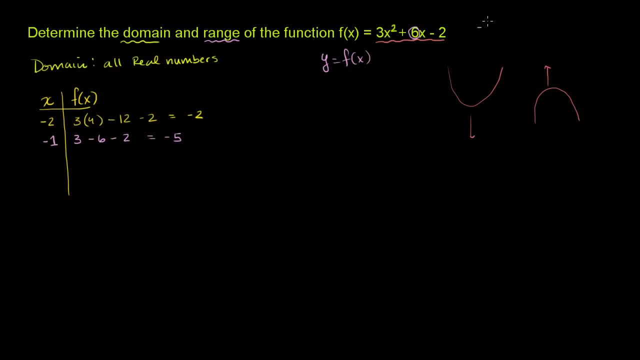 So negative b, that's the coefficient on this term. right over here It's negative 6 over 2 times this one right over here, 2 times 3.. This is equal to negative 1.. So that is the vertex, But let's just keep on going right over here. 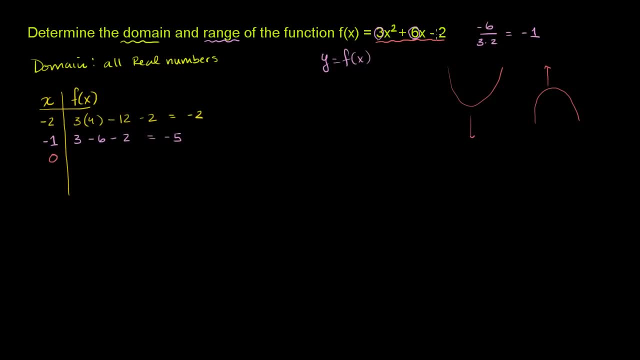 So what happens when x is equal to 0? These first two terms are 0. You're just left with a negative 2. When x is equal to positive 1, and this is where you can see that this is the vertex. 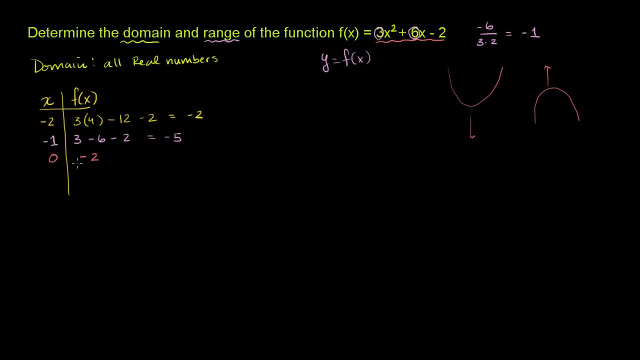 And you start seeing the symmetry: If you go 1 above the vertex f of x is equal to negative 2.. If you go 1 x value below the vertex or below the x value of the vertex f of x is equal to negative 2 again. 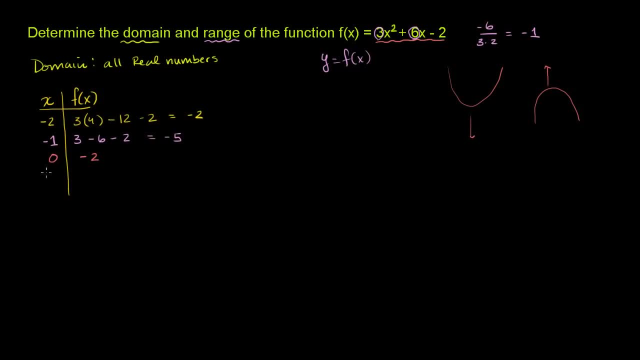 But let's just keep going. We could try. let's do one more point over here, So we could try. x is equal to 1.. When x is equal to 1, you have 3 times 1 squared, which is 1.. 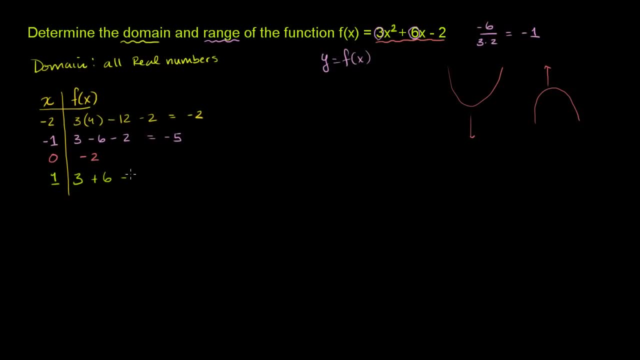 So 3 times 1 plus 6 times 1,, which is just 6, minus 2.. So this is 9 minus 2.. It's equal to 7.. And that, I think, is enough points to give us a scaffold of what this graph will look like. 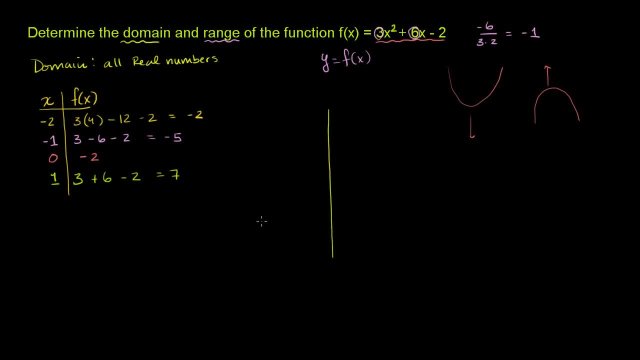 what the graph of the function would look like. So it would look something like this: Let me do my math. I'll do my best to draw it. So this is: x equals negative 2.. Let me draw the whole axes. This is: x is equal to negative 1.. 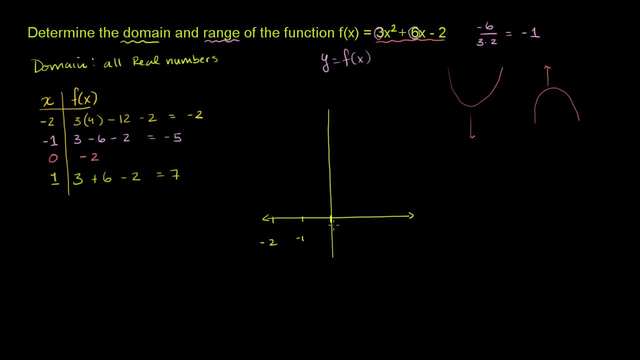 This is x is equal to 0. And then this is x is equal to 1, right over there. And then when x is equal to, we go from negative 2 all the way to positive, or we should go from negative 5. 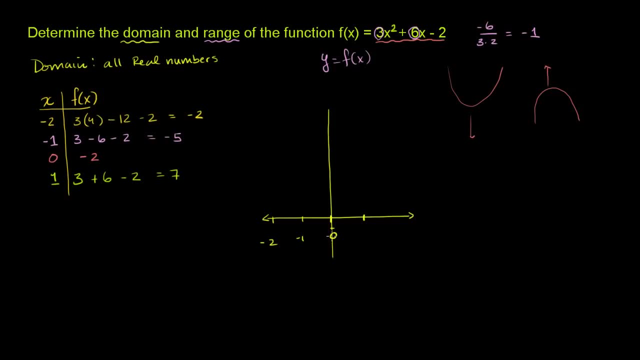 all the way to positive 7.. So let's say this is negative: 1,, 2,, 3., 4, 5. That's negative 5 over there on the y-axis. And then let me go to positive 7.. 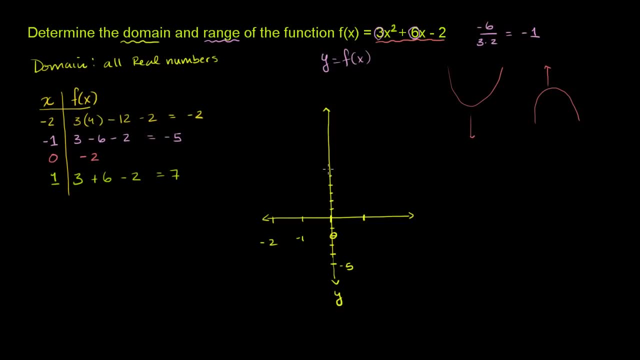 1,, 2,, 3,, 4,, 5,, 6, 7.. I could keep going. This is in the y And we're going to set y equal to whatever our output of the function is. y is equal to f of x. 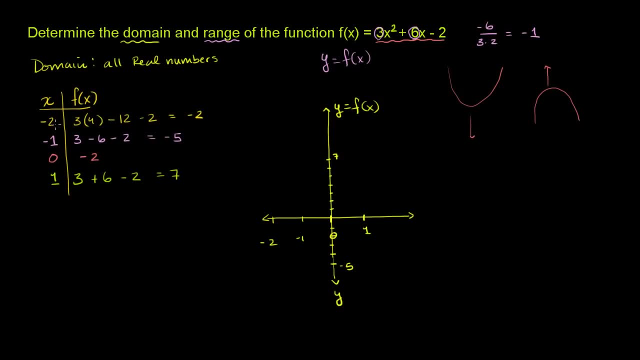 And this is 1 right here. So let's plot the points. You have the point: negative 2, negative 2.. When x is negative 2, this is the x-axis. When x is negative 2, y is negative 2.. 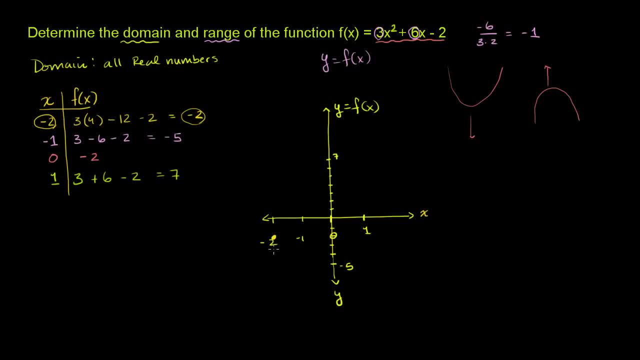 So that is that right over there. So that is the point. negative 2 comma, negative 2.. Fair enough, Then we have this point. We have this pink or purplish color When x is negative 1, f of x is negative 5.. 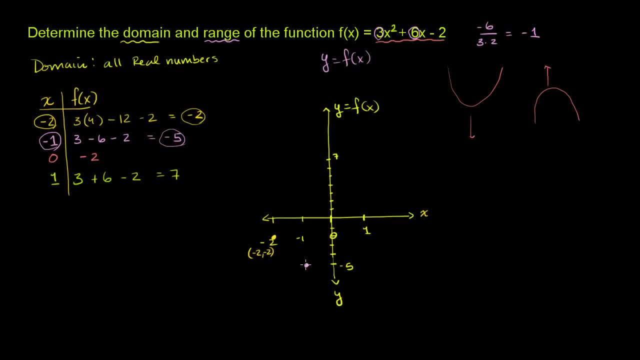 When x is negative 1, f of x is negative 5.. And we already said that this is the vertex, And you'll see the symmetry around it in a second. So this is the point 1, negative 5.. And then we have the point 0, negative 2.. 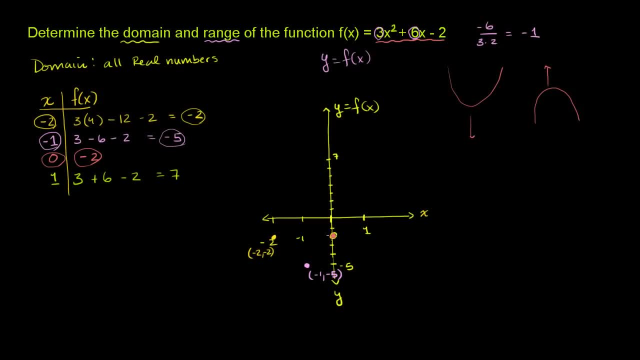 When x is 0, y is negative 2.. Or f of x is negative 2.. Or f of 0 is negative 2.. So this is the point: 0, negative 2.. And then, finally, when x is equal to 1, f of 1 is 7.. 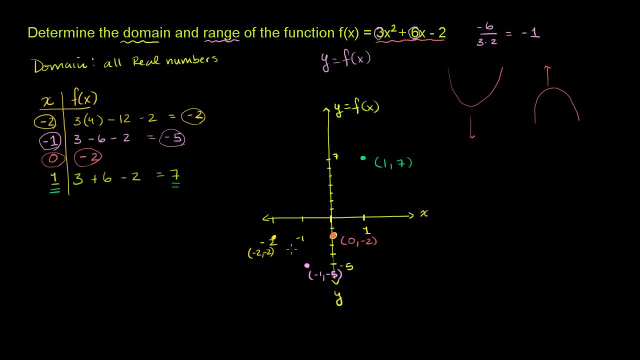 So that, right, there is the point 1, comma 7.. And it gives us a scaffold for what this parabola, what this curve, will look like. So I'll try my best to draw it respectably, So it would look something like that: 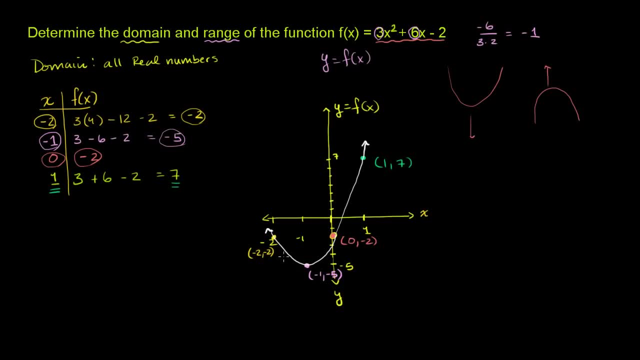 And keep on going in that direction. keep on going in that direction. But I think you see the symmetry around the vertex That, if you were to put a line right over here, the two sides are kind of the mirror images of each other. 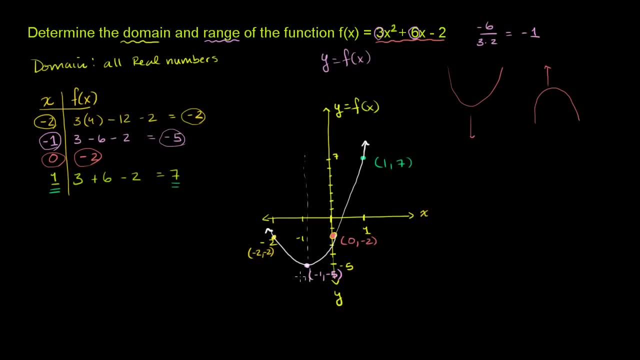 You can flip them over, And that's how we know. it's the vertex And that's how we also know, because this is an upward-opening parabola. I mean, there is formulas for vertexes and there are multiple ways of calculating it. 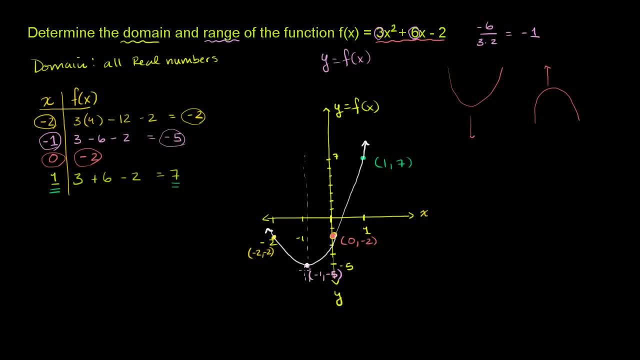 But since it's an upward-opening parabola, the vertex is going to be the minimum point. This is the minimum value that the parabola will take on. So, going back to the original question, this is all for trying to figure out. 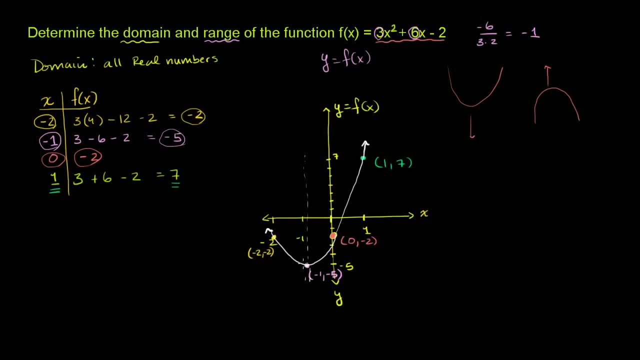 the range, the set of y values, the set of outputs that this function can generate. You see that the function it can get as low as negative 5.. It got all the way down to negative 5 right at the vertex, But as you go to the right, as x values increase to the right. 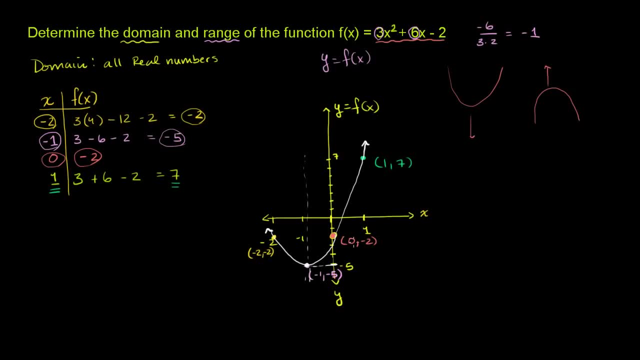 or decrease to the left, Then the parabola goes upwards. So the parabola can never give you values. f of x is never going to be less than negative 5. So our domain, but it can take on all the values. 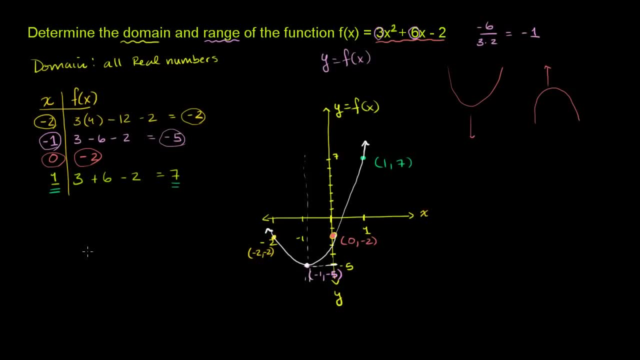 It can keep on increasing forever as x gets larger, x gets smaller away from the vertex. So our range here- so we already said the domain- is all real numbers. Our range, the possible y values, is all real numbers greater than or equal to negative 5.. 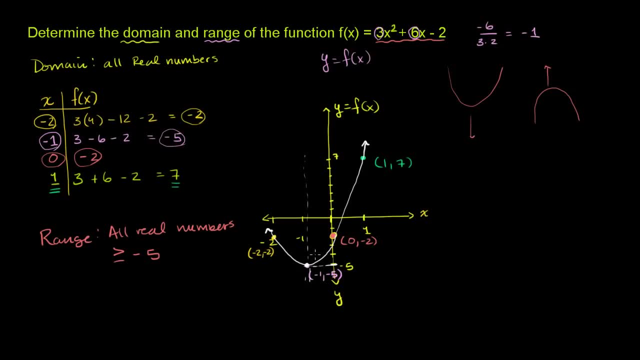 It can take on the value of any real number greater than or equal to negative 5, nothing less than negative 5.. 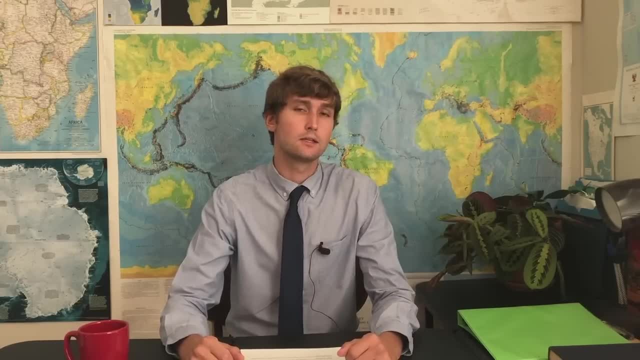 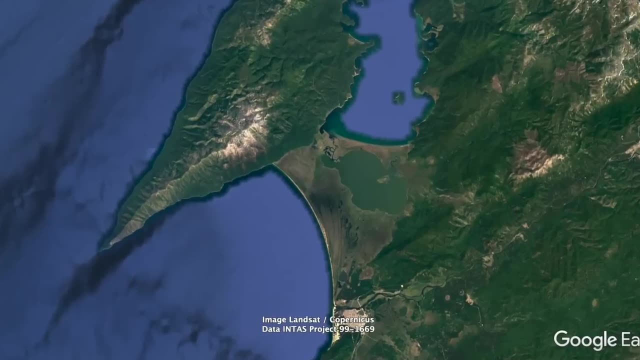 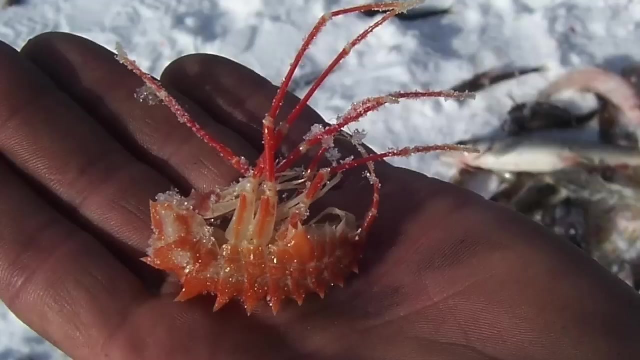 Like other great lakes in North America and Africa, Lake Baikal is truly an inland sea, complete with a wide range of environments, From surf zones, rocky cliffs and river estuaries to underwater canyons. It has its own species of sponge, weird deepwater invertebrates. 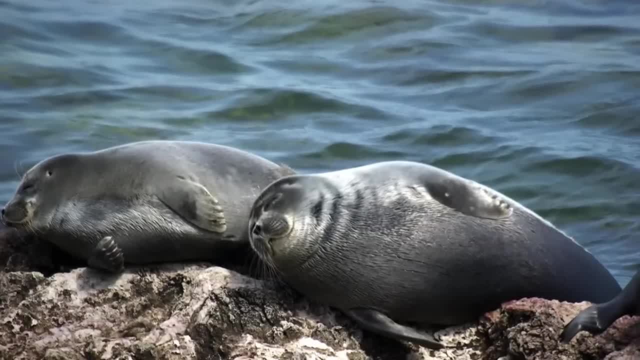 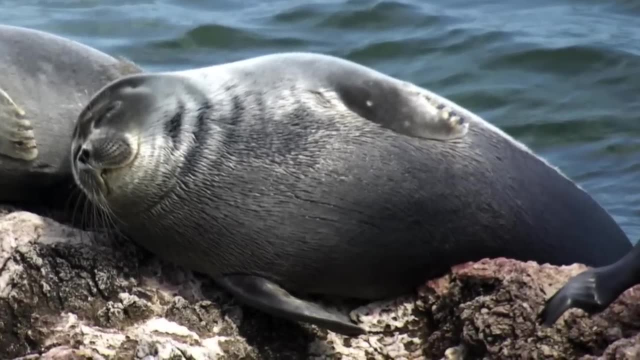 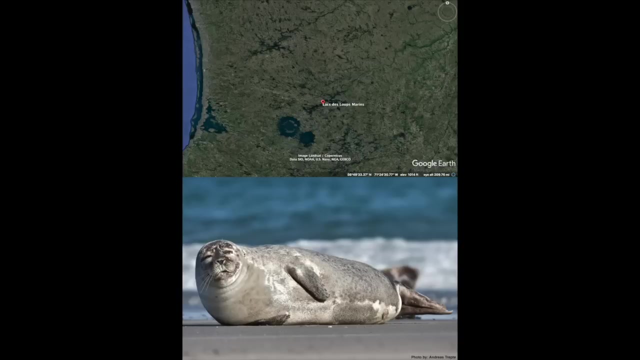 and endemic fish, But perhaps most fascinating is the Baikal seal, or nerpa, the world's only entirely freshwater species of seal. There are populations of freshwater seals elsewhere: The ringed seals of Lake Ladoga in Russia, the Ungava seal, a harbor seal that inhabits 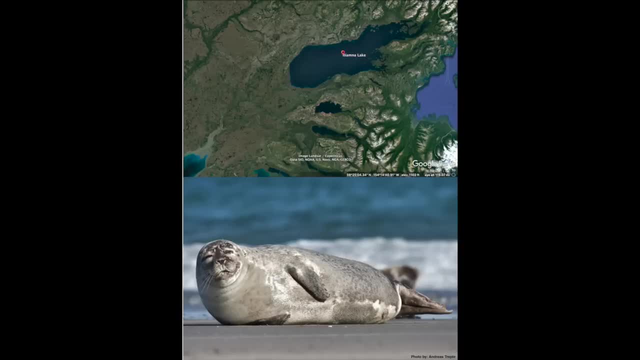 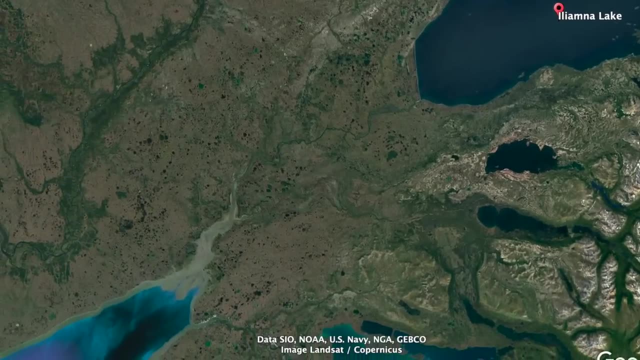 freshwater lakes in Quebec and the harbor seals of Iliamna Lake in Alaska are three other examples. But it's easy to imagine how these seals colonized the lakes. The ocean is right next door. How on earth did seals get to Lake Baikal Somehow? 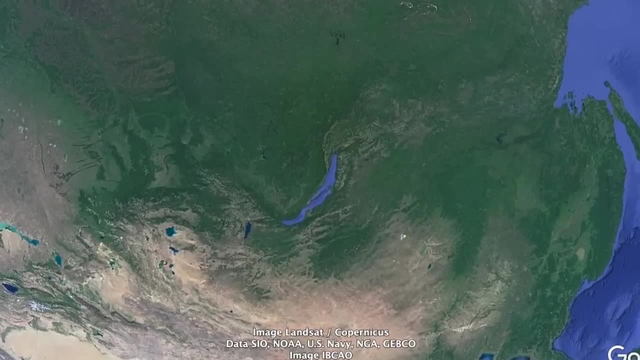 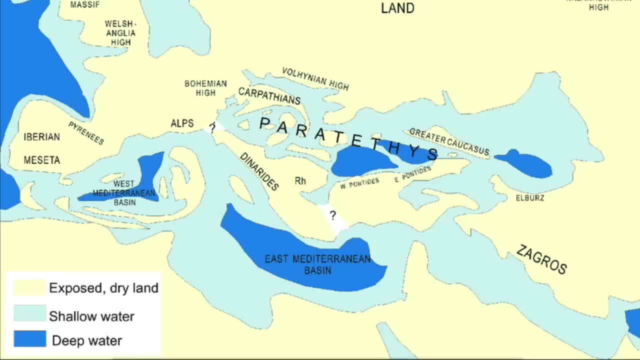 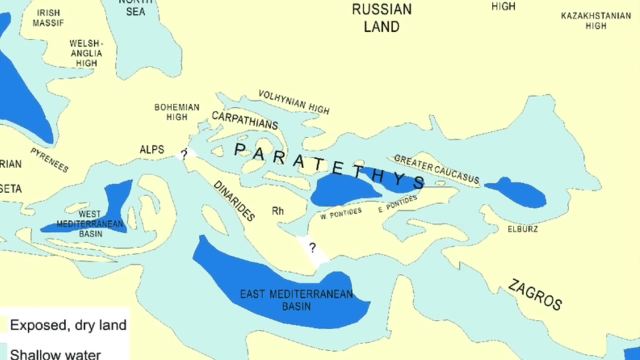 somewhere the ancestors of the Baikal seal managed to reach the center of the Asian continent. Based on current evidence, just how did they manage to do it? An outdated idea was that Baikal seals and Caspian seals, who were also isolated from the greater ocean, became trapped in the 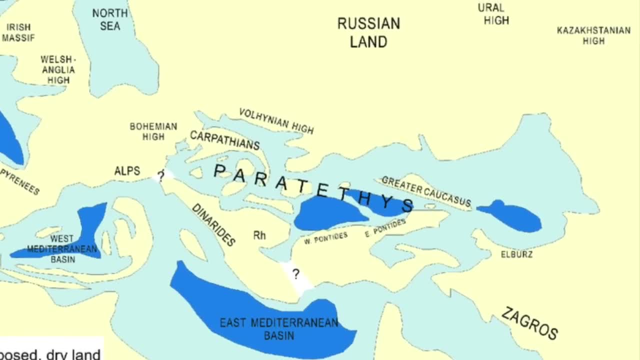 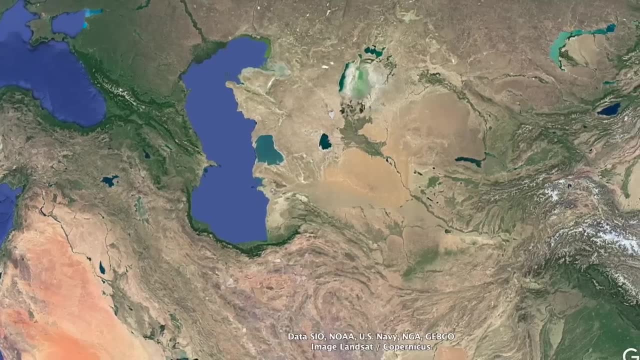 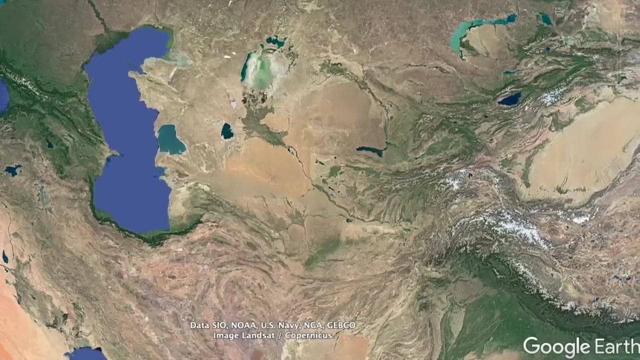 interior of Asia. back before the Miocene, when a vast arm of the Mediterranean, the Paratethes, stretched into the heart of the continent, The seals became isolated, according to this theory, as tectonic forces and a drying climate isolated the Caspian Sea and other bodies of water. 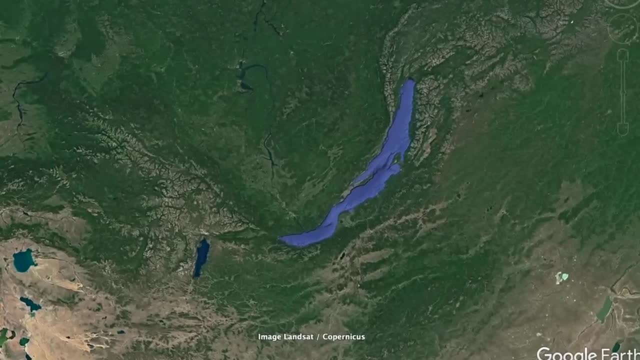 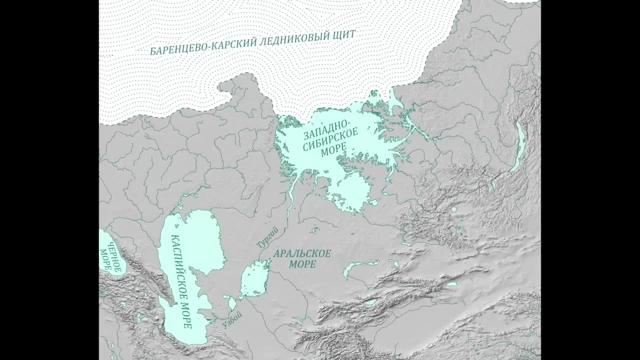 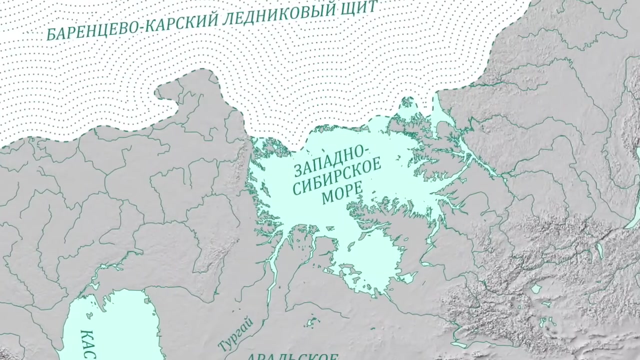 The Paratethes wasn't connected to Lake Baikal, but it did bring seals much closer to the lake than any ocean connection today. A more widely supported theory was that arctic seals in Siberian estuaries became trapped by ice sheets during glacial periods and huge lakes formed in front of the ice.